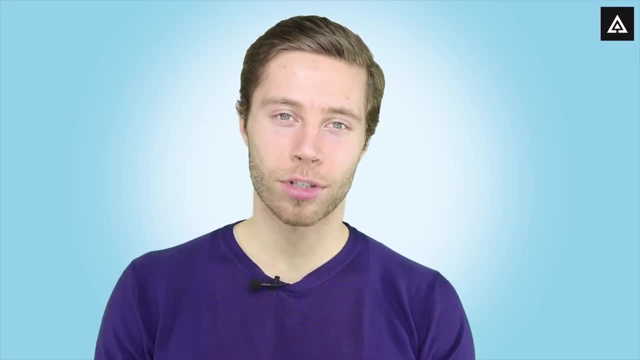 Hey guys and welcome back to my channel. that is all about artificial intelligence, blockchain and technology in general. Today, we're going to talk about overfitting in machine learning. What is it? Something that a lot of you people probably are wondering, So let's get into it In general, you. 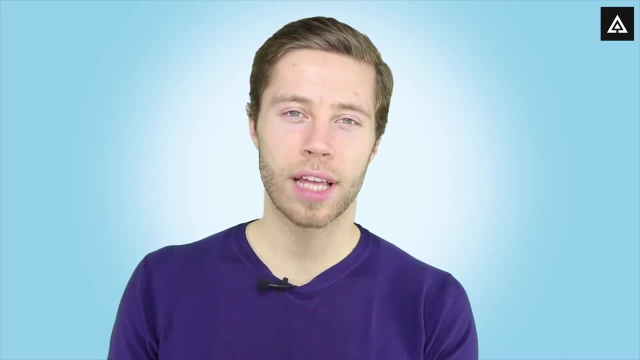 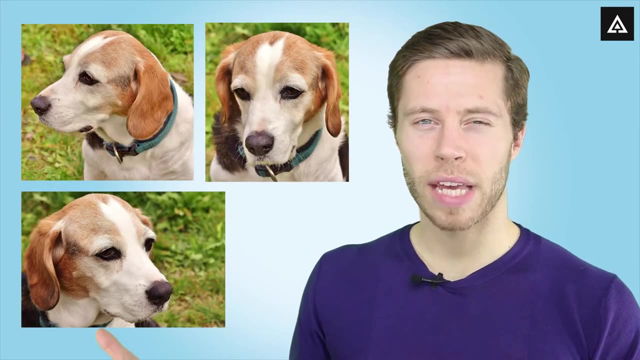 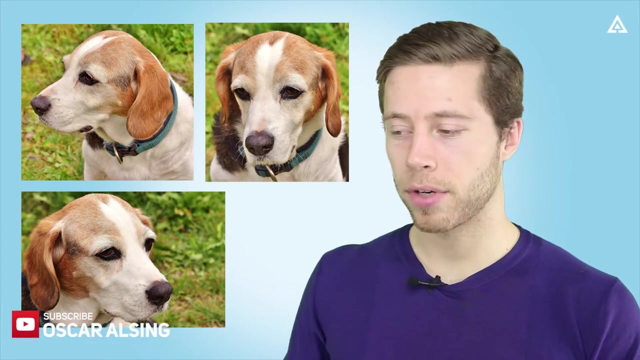 can say that overfitting is when you have a model that tries to adapt itself too much to the data that you have. So, for example, let's have a look at these dogs here. You see they all are quite the same, right? They all look very similar. What happens then when you have a very complex model, a very 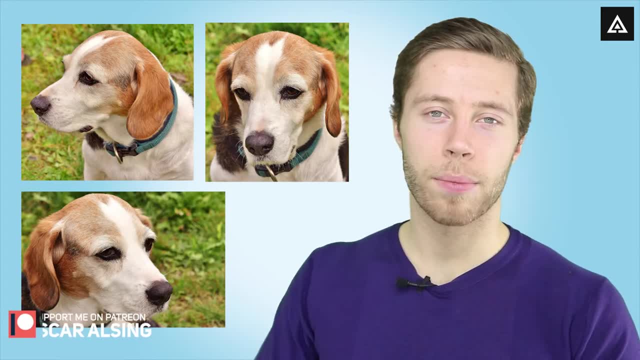 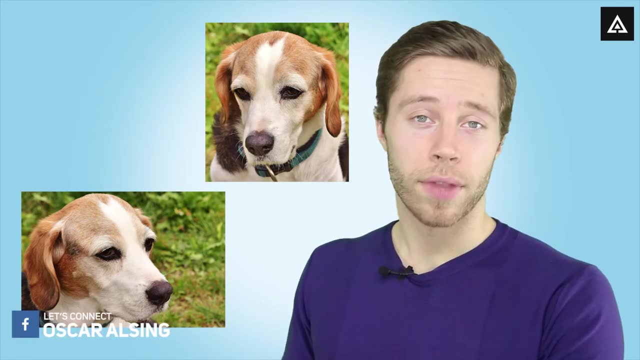 advanced model, a model that has a lot of neurons, for example, that wants to be able to distinguish. if it is a dog on a picture And this is all the training data that it has, Then a possible problem could be when our model sees this image. It's still of a dog, right, But it looks very different from. 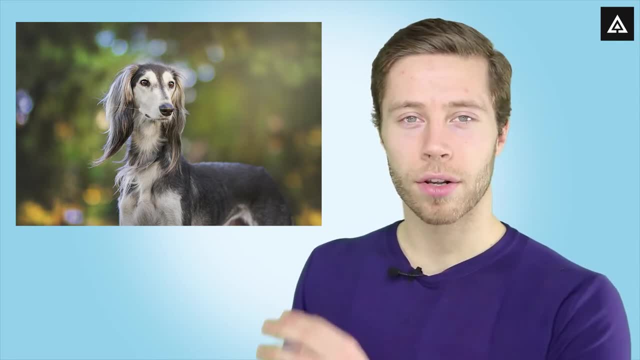 the other dogs, And our model here has just learned to mimic the other dogs and what they look like. So when it sees an image, it can see whether it is a dog or not. So this is a model that is used to see the other dogs. 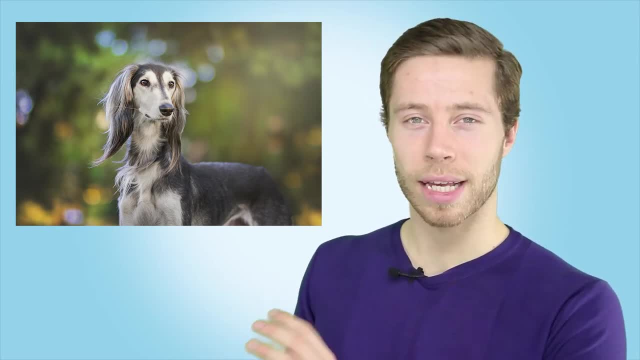 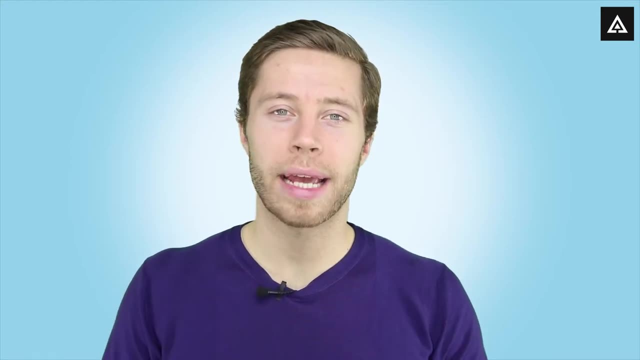 of another dog. it doesn't really know that it is a dog because it doesn't look exactly the same as the other one, and this is a big problem in machine learning. i do think that you now have a broad perspective on what overfitting actually is, so i encourage you to hit the like button down here to 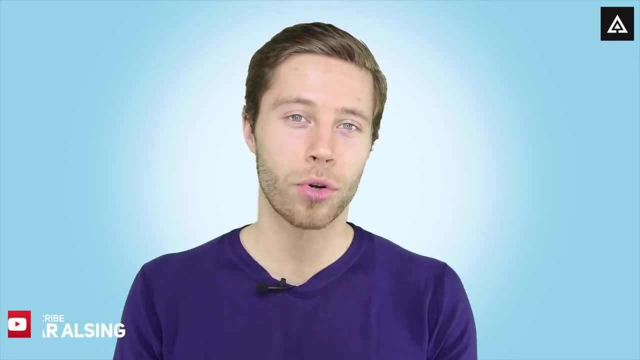 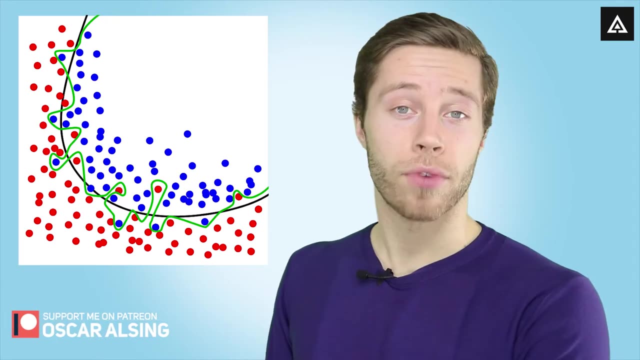 your right to actually, you know, make some sound of joy, as you now know what overfitting is. but let's dive deep a bit more and look at some graphs. if you take a look at this graph here, you can see that we have red dots and blue dots. these two dots represent two different classes, and that's. 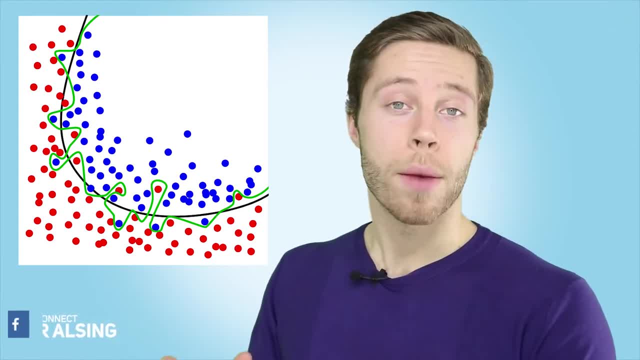 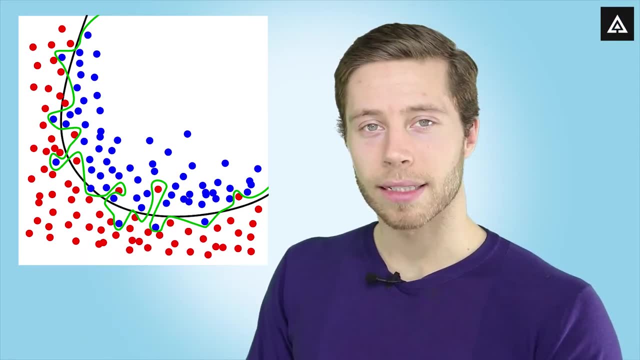 why they have different colors. you can think of them as cats and dogs, or male or female. in this very case, we have two lines, we have the black line and we have the green line. and these lines- you can think of them as the machine learning model that tries to distinguish between the two different 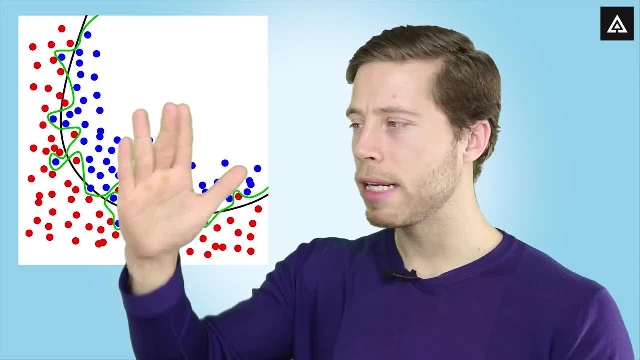 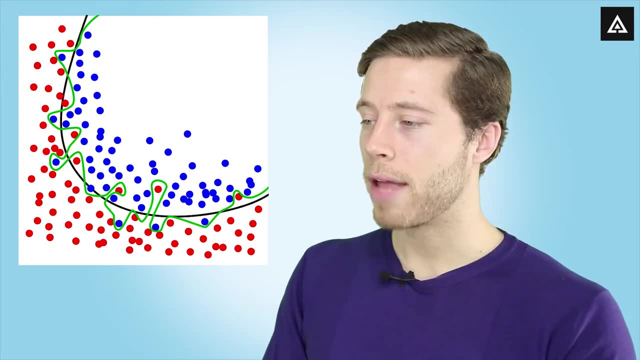 classes. as you see here, the green line really follows the data we have here, the training data, the data that we get access to in order to learn this data pattern, and the black line is a bit more smooth. as you also can see, the green line never is wrong.